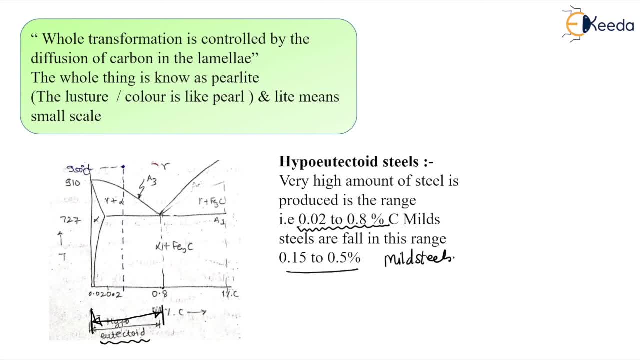 Now, dear students, again I am going below, above this A3 line, that is, everything is gamma, here again at 950 degree centigrade, And I have chosen the percentage of carbon as 0.3% of carbon. So at 0.3% of carbon at 950 degree centigrade, if you see. 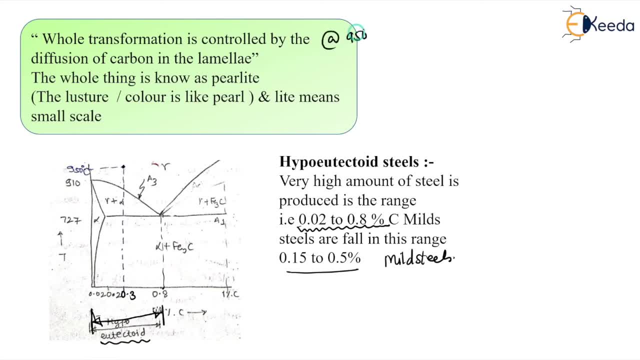 So at 950 degree centigrade, dear students. So everything will be what? So everything will be what. The gamma isn't it? Because there is only gamma, Gamma, austenite. Now, dear students, as soon as I come below this A3 line, 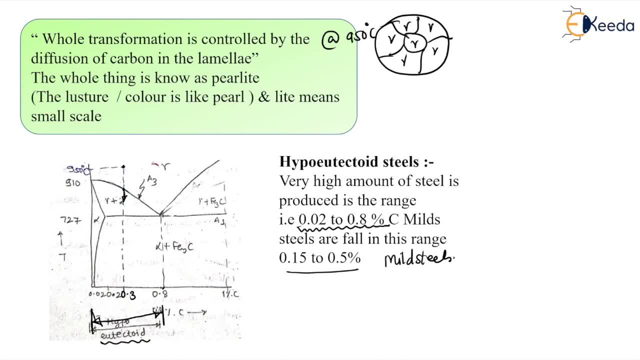 So below A3 line, as here is what, Near to gamma, This is alpha rich region, isn't it? Definitely So below this A3.. Some gamma will getting transformed to this alpha at the grain boundaries, dear students. See, when I come below this A3 line, 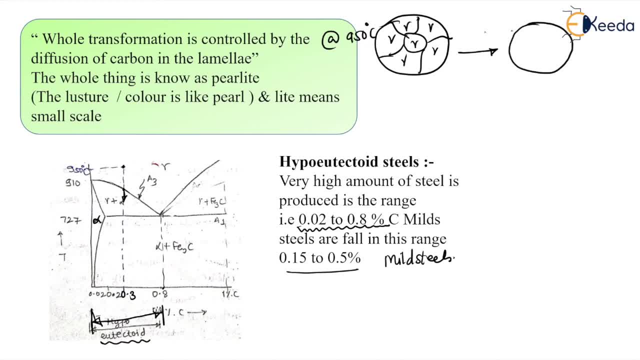 So some of this gamma, which is already present here in this microstructure, Now at the grain boundaries, It will going to transform, Say, it will going to transfer into what Alpha Say. this is the alpha, dear students At the grain boundaries, this gamma, 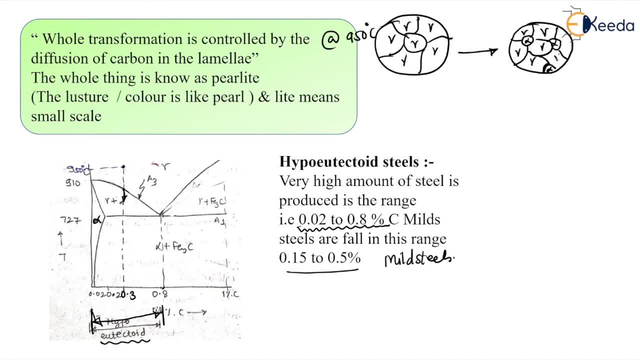 This gamma is transforming into this alpha At the grain boundaries, At the, of course, at the grain boundaries. So, dear students, as we know that alpha does not require any carbon, isn't it? Therefore, the gamma region is get enrich in the carbon, isn't it? 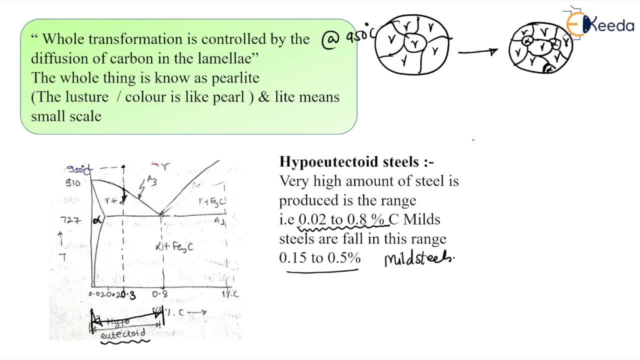 So here now, some gamma which is left over become transformation is low, isn't it So, if you see below this A1 line now. So whatever the transformations of this, some gamma austenite Below A3 into the alpha at the grain boundaries, 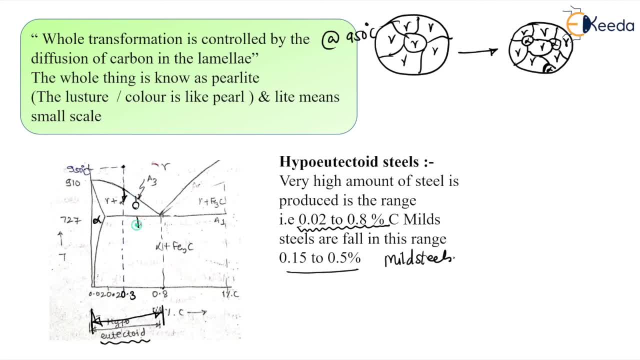 Now below this A1 line, below this A1 line. So all gamma grains going to transfer into what? This alpha plus Fe3C, into the layer by layer structure. That is the lamellage, isn't it? And the structure is pearlite, isn't it? 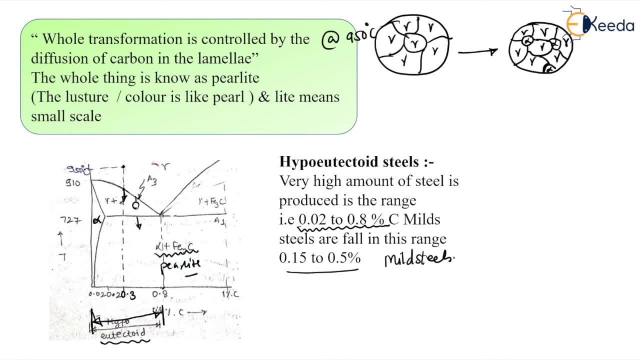 But, dear students, in this pearlite also This, some alpha get retained on this grain boundaries, isn't it? So if I draw the microstructure below A1 line, Below A1 line, So what you are going to see? So below A1 line. 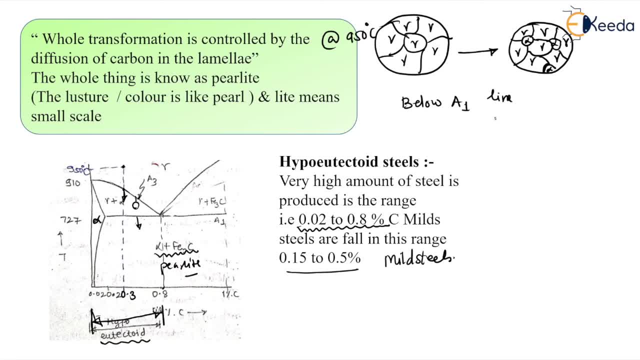 This gamma will be no more there. Now, gamma is going to transform into what? The lamellage of alpha and cementite. isn't it, Alpha and cementite? But at the grain boundaries, some alpha is going to retain. This alpha is going to retain. 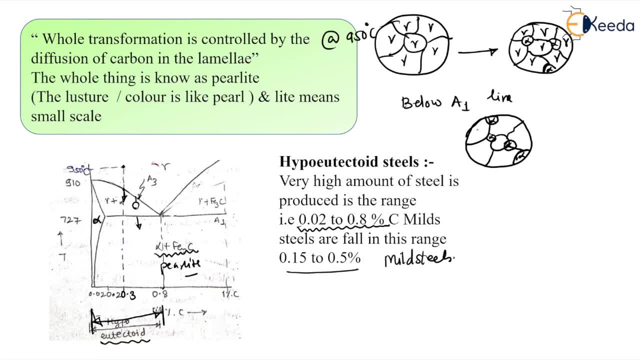 And left over. And left over will be what? When this cooled below the A1 line, We will be having this, layer by layer, structure of what This? alpha and cementite, Alpha and cementite. So, dear students, I am showing this black color with the cementite. 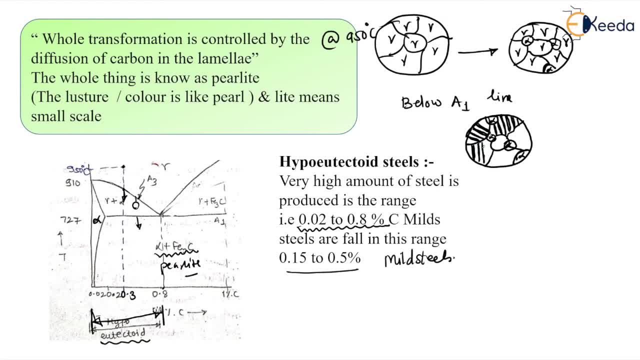 And definitely I will show with the red color That is the alpha. So I will show this alpha here. Like that, you will be having again our pearlite, isn't it? And at the grain boundaries, definitely there will be the alpha, Which is get retained, isn't it? 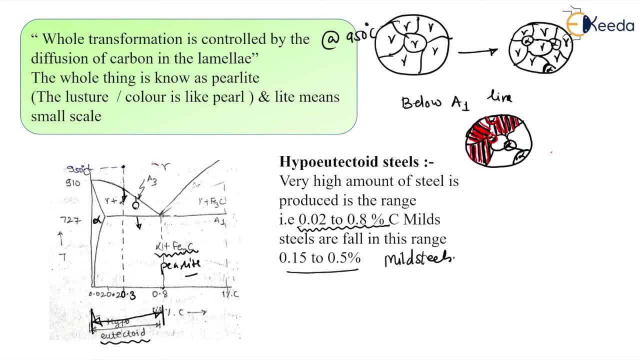 So, dear students, this alpha are bigger, isn't it? Whatever this alpha which is get on this grain boundaries, Which the gamma is transformed into, this alpha, They are generally big And because of this alpha is bigger in nature, It will have a very good ductility. 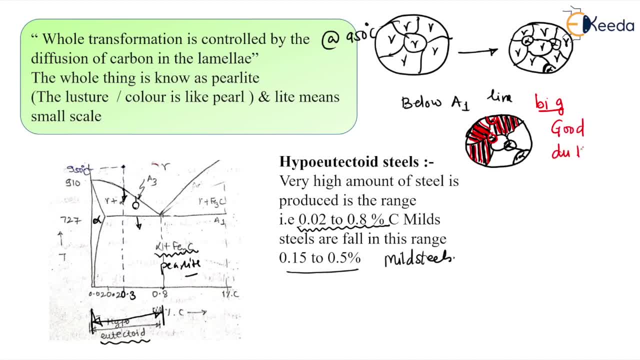 It will have very good ductility. And, dear students, now see here One alpha you can see here, at the grain boundaries Where this gamma is transformed into the alpha. And one alpha you can see in the layer by layer structure of this pearlite. 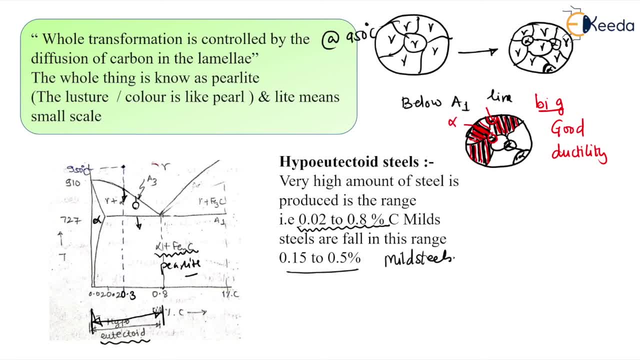 That is, this red color is alpha And black is cementite Fe3C. So, dear students, you are having in this microstructure of this hypo eutectoid steels, Below a one line you will be seeing, There will be the alpha, which is in the laminar. 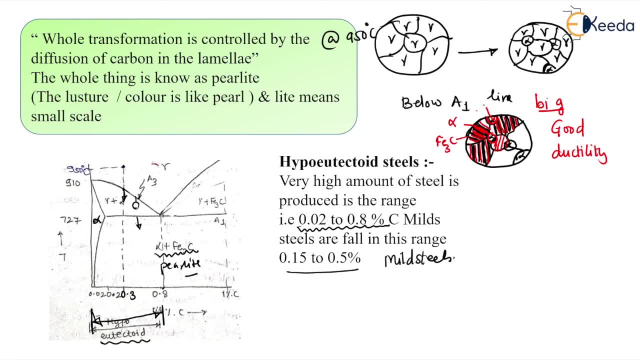 Which is in the layer form, And one alpha which is at the grain boundaries. isn't it So, dear students? The alpha which is present on this grain boundaries, Which is bigger in nature, This is called it as pro eutectoid. 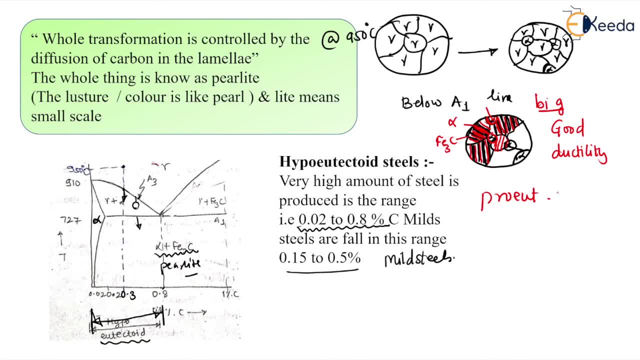 Pro eutectoid alpha, dear students, And the alpha which is present in the layer form Alpha, which is present in the layer form In the lamellies, Is known as the eutectoid alpha. The eutectoid alpha, dear students. 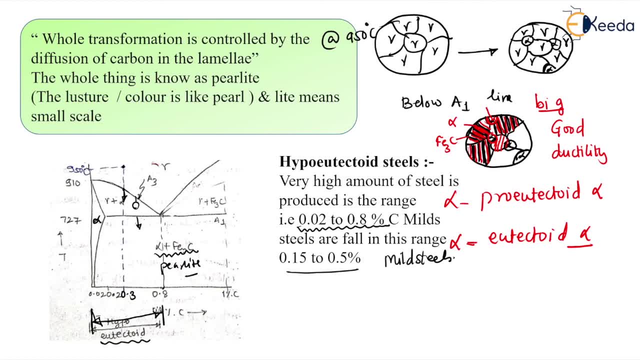 So this is how this transformation, dear students, is occurring. So, in short, what you can say: We have taken 0.3% of carbon And we are going into 950 degree centigrade, Where everything was gamma austenite. Now we started cooling that gamma austenite. 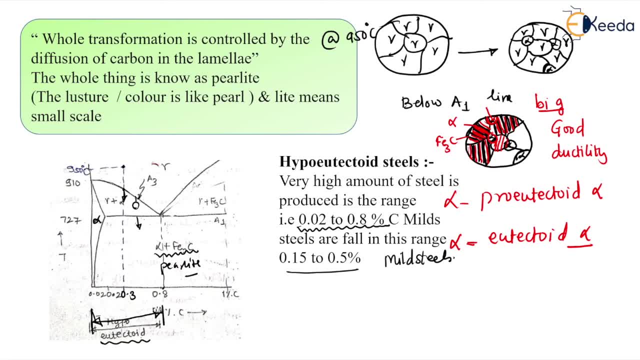 So when we just come below this A3 line, So because of this alpha rich region, So definitely there will be the nucleation of alpha. So nucleation means actually what I cannot say: the nucleation, But here some of this gamma which is present in the grain. 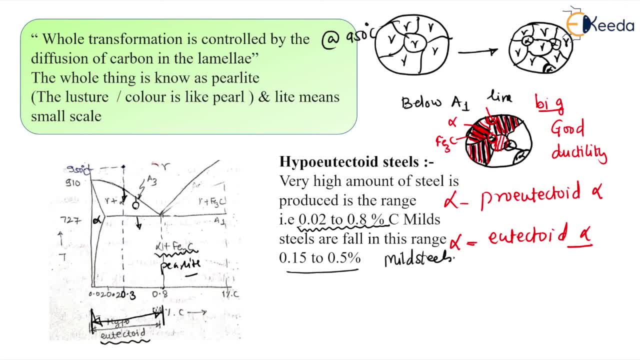 Which get converted into the alpha, Get transferred into the alpha, Where, At the grain boundaries, here At the grain boundaries, it get transferred into alpha And when definitely we come below this A1 line, A1 line, We are having definitely here the pearlitic. 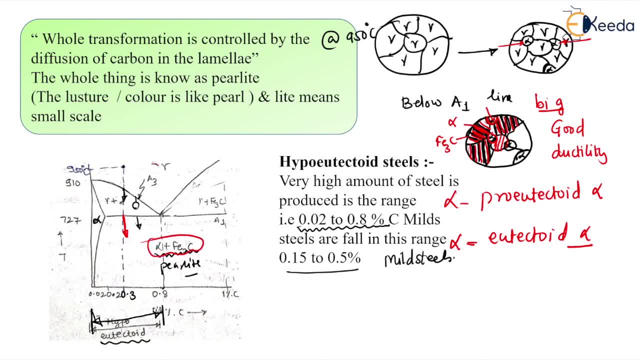 Where there are the layers of alpha and cementite. Alpha and cementite. So this is how we can get here in the microstructure: One alpha at the grain boundaries And one alpha in the form of layer. So alpha, which is at the grain boundaries, 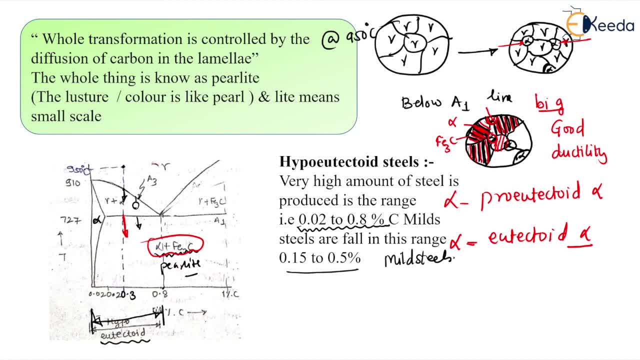 Is bigger, Gives good ductility for the steel, And that alpha is known as the pro eutectoid alpha, dear students. And the alpha which is present in the layer Is known as the eutectoid alpha, Isn't it? 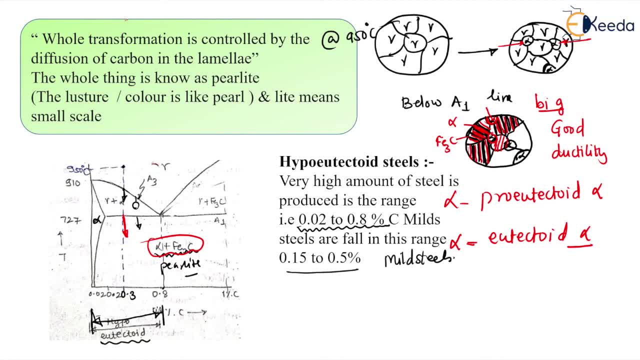 So this is how, dear students, This hypo, This hypo eutectoid, Eutectoid transformation is happening. Transformation We have seen. Okay, So this is a hypo eutectoid transformation, dear students. So, dear students, in next video, 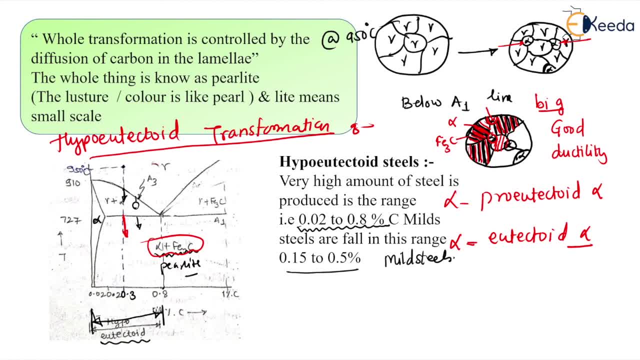 We are going to see about this Hyper eutectoid transformation. That will be the last transformation In this iron and iron equilibrium diagram, Dear students, So thank you so much for seeing this video.